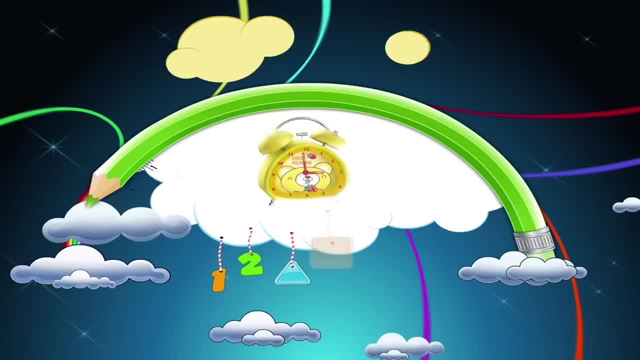 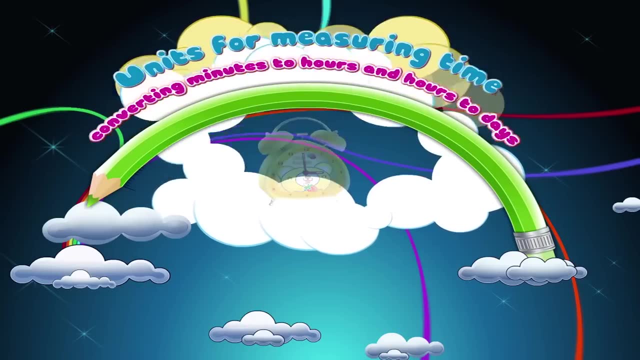 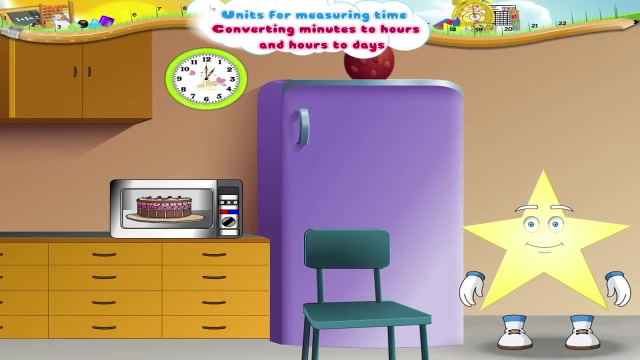 Units for Measuring Time. Starry surprise, There's a cake getting baked for you. Oh, you can smell it, But you will have to wait for an hour before you eat it. Why do you keep looking at the clock? starry? 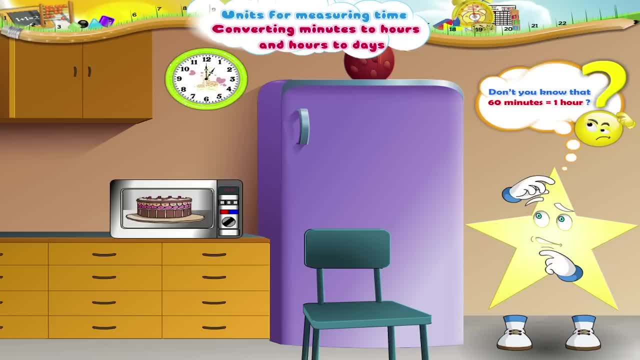 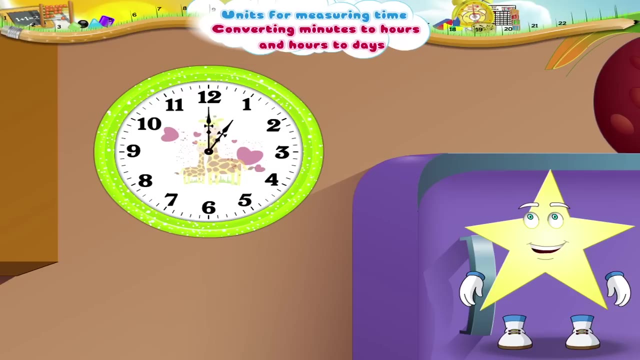 There's still plenty of time. Don't you know that 60 minutes make an hour? I understand you have forgotten your time measurements. Let me revise them with you. Here is a clock, starry. As you know, it has an hour hand. 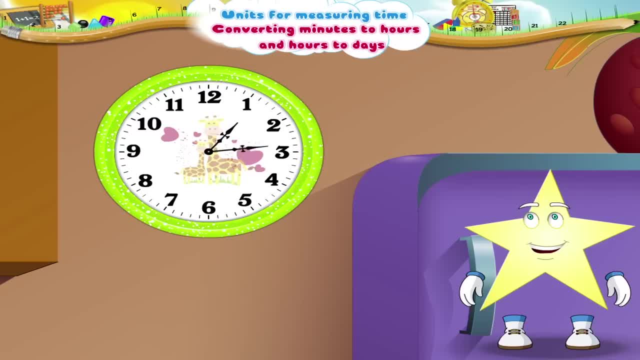 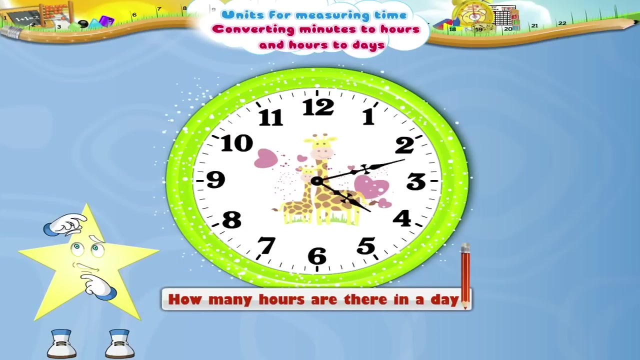 and a minute hand that keeps turning throughout the day, telling us the time. Now, do you know how many minutes make an hour? starry, Yes, 60 minutes make an hour. And how many hours are there in a day? starry, Right, 24 hours make a day. 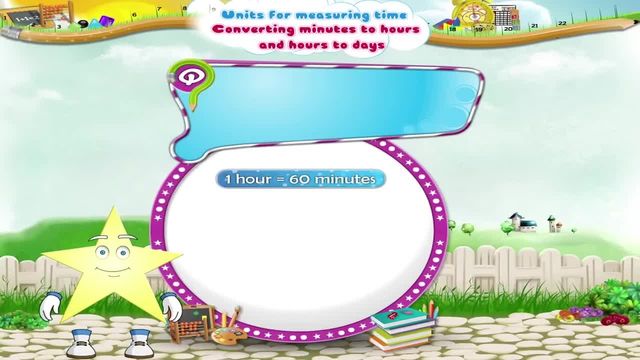 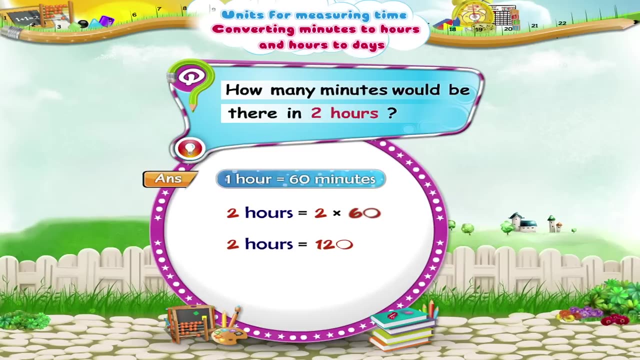 Starry, if one hour has 60 minutes, how many minutes would be there in 2 hours? We would have to multiply 2 by 60. Which is 120 minutes. So 2 hours would be equal to 120 minutes. 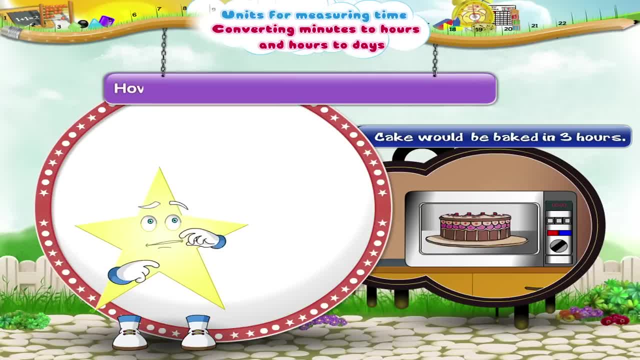 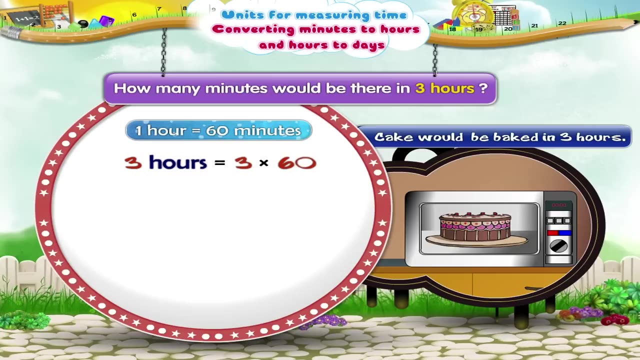 Now suppose the cake would take 3 hours to bake. How many minutes would that be? Let us work it out: 1 hour equals 60 minutes, So 3 hours will be 3 multiplied by 60. Which is 180 minutes. 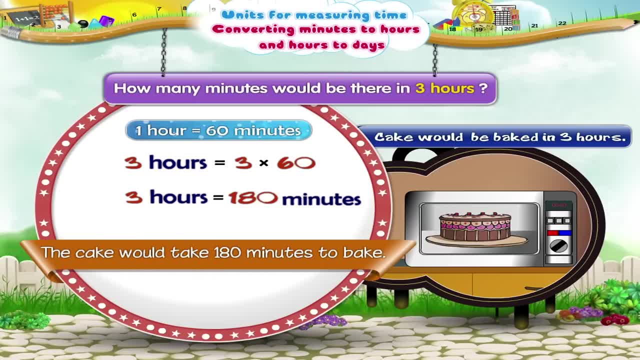 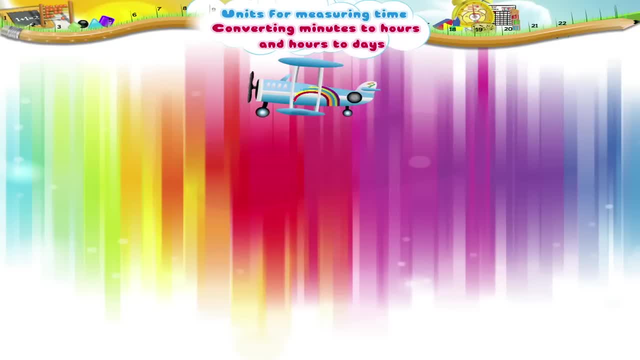 The cake would take 180 minutes to bake. 1 hour equals 60 minutes. So 3 hours will be 3 multiplied by 60. Which is 180 minutes. The cake would take 180 minutes to bake. 1 hour equals 60 minutes. 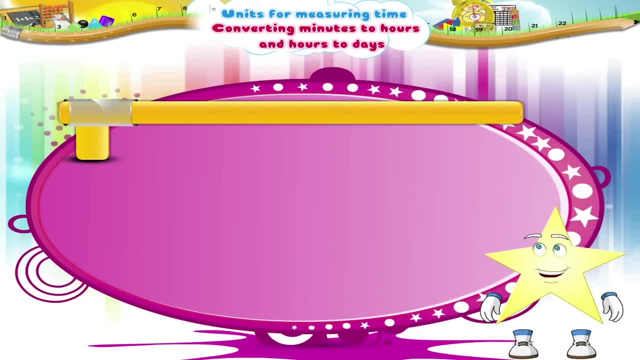 Since we know that 24 hours make one day story, let us find out how many hours are there in two days. One day equals 24 hours. Two days means 2 multiplied by 24, which is 48 hours. Two days has 48 hours. 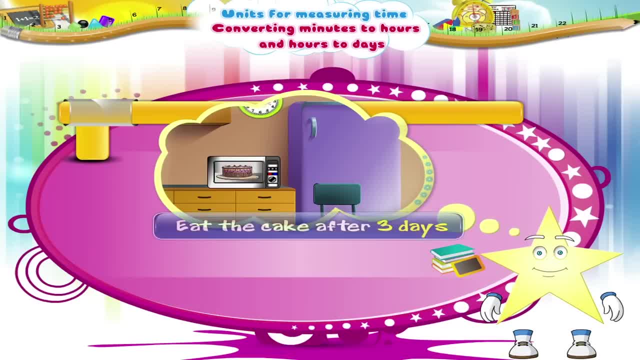 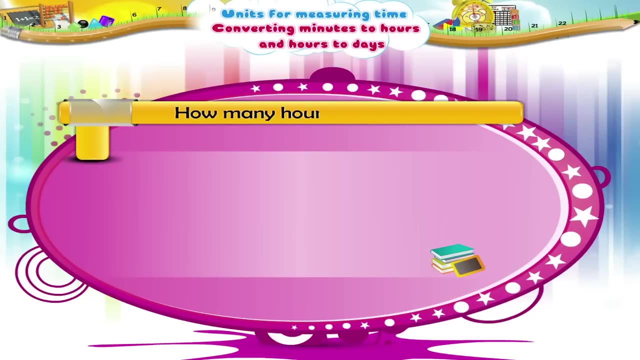 Starry, if you are told not to eat the cake for three days, after how many hours would you be able to eat the cake? You're still thinking: Wait, I'll explain How many hours in three days? Now, one day equals 24 hours. 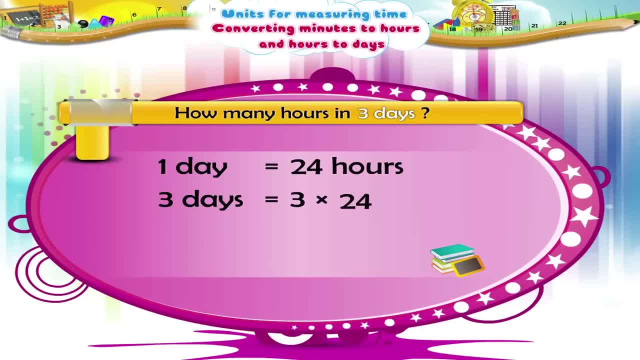 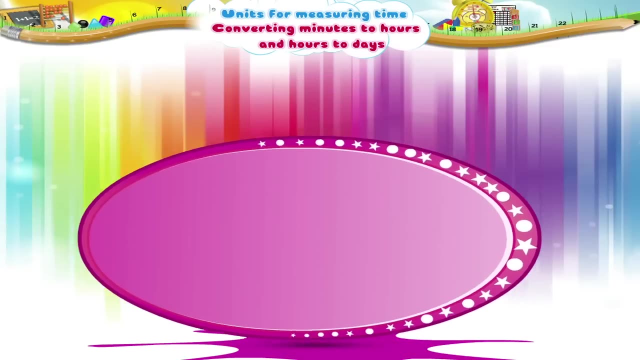 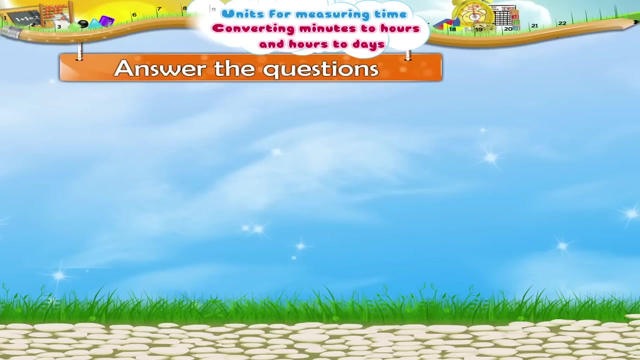 Three days. That means 3 multiplied by 24, which is 72 hours. You will be able to eat the cake 72 hours later. Now let us revise what we have studied. One hour has dash minutes. One hour has 60 minutes. 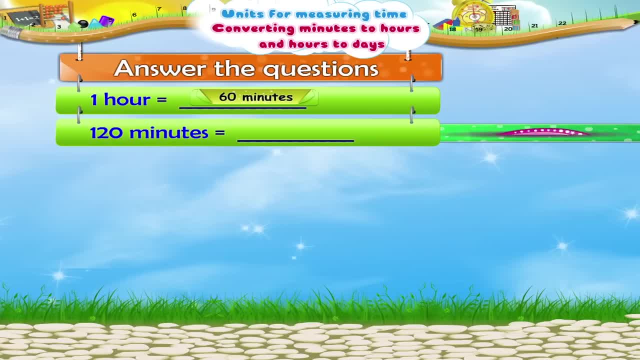 There are 120 minutes in dash hours. There are 120 minutes in two hours. One day has dash hours. One day has 24 hours. One day has 44 hours. One day has 24 hours. One day has 25 minutes. 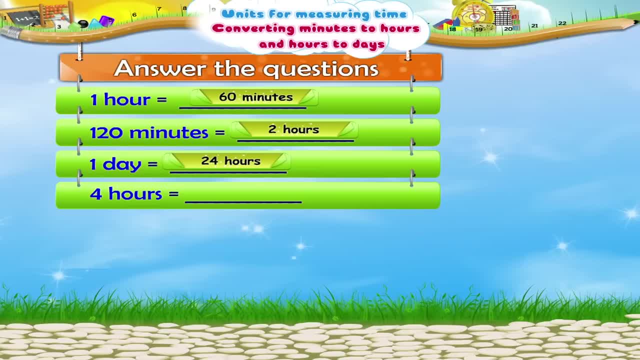 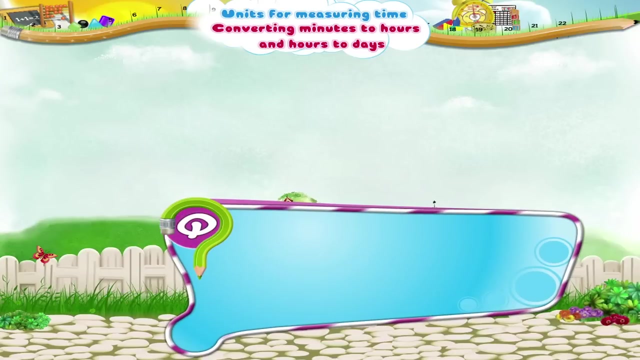 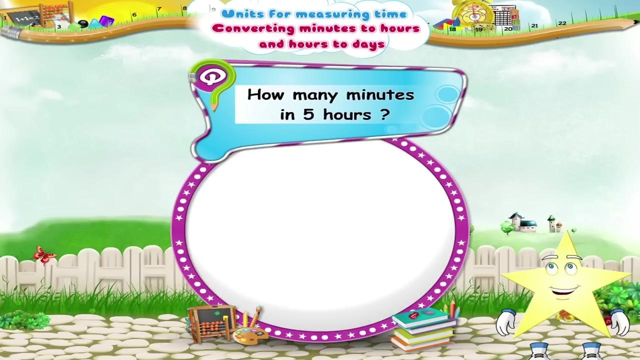 Four hours. Four hours means dash minutes. Four hours means 240 minutes. There are dash hours in two days. There are 48 hours in two days. Now solve these problems. How many minutes in five hours? Five hours equals five multiplied by 60, which equals 300 minutes.